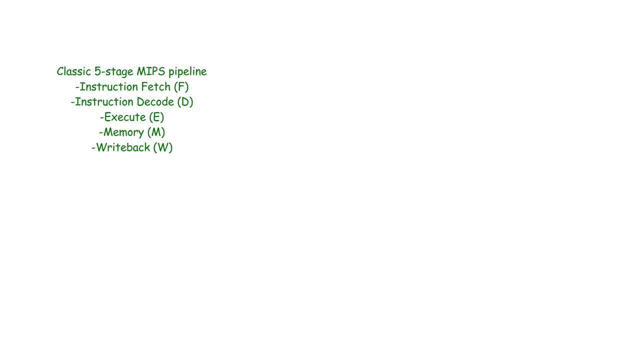 for each of these stages is shown in parentheses, And so, to make this concrete, we want to look at a specific example, and the code for the example we're going to look at is shown here, And so this is the high-level C code for it, and this is a loop that is going to execute 100 times Each. 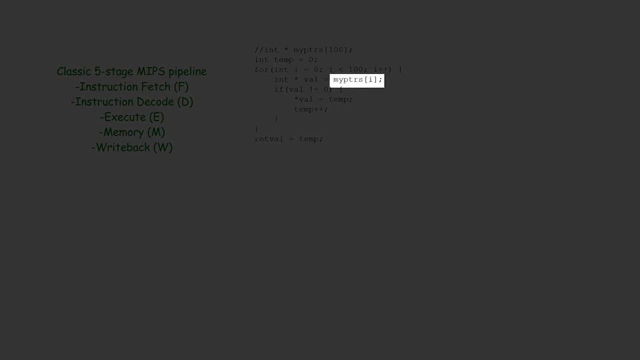 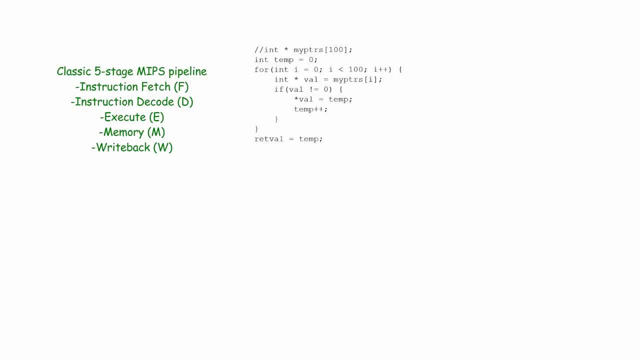 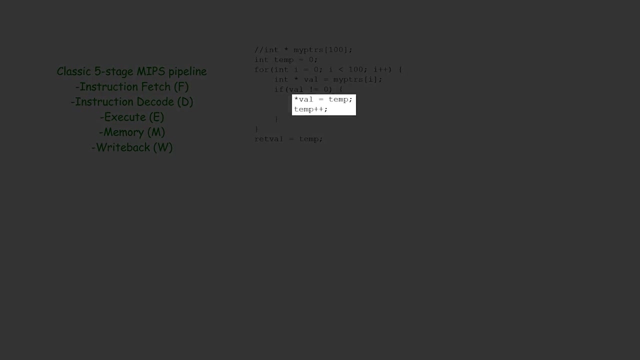 time through the loop, we're going to load the value from an array and we're going to interpret this value as an address or a pointer to some location in memory. If this pointer is non-zero- meaning it has a legitimate address- then we're going to assign to this address a value that we 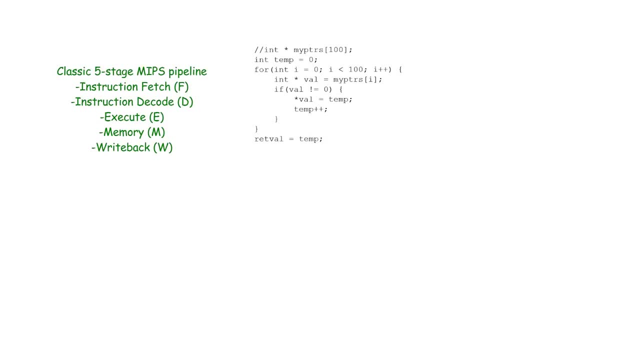 are going to increment for each legitimate value we find And then at the end we're going to have a count of the total number of non-zero addresses that we found, as well as having assigned each of those addresses to its index through. of the legitimate values, There are a: 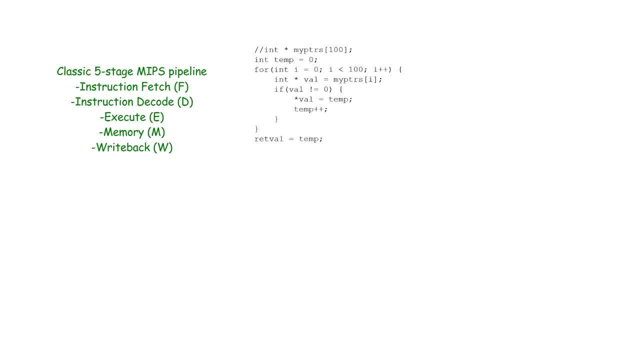 number of different ways that this could be converted into MIPS assembly. The one that we're going to look at is shown here and of primary interest is this region highlighted, where that shows the 10 instructions that make up the loop and the ones that are going to be executed. 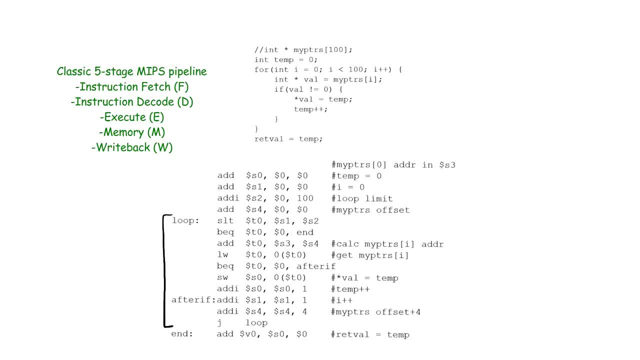 repetitively as this loop is executed. And so I will note, in this example we're going to be assuming a slight variation on MIPS assembly. So, while true MIPS assembly has a branch delay slot, in this example we're going to follow. 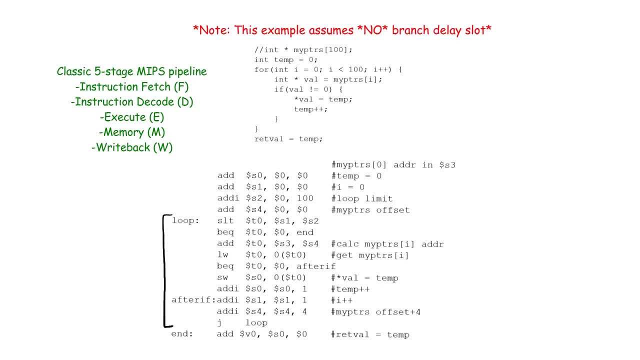 the convention of many textbooks on the field, where we assume there is not a branch delay slot. So this means the instruction after a branch or a jump is not expected to be executed unless the branch is not taken. Within this code there are two branches and so we want to consider how the 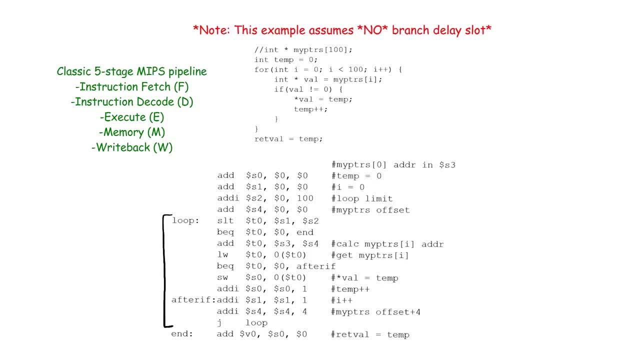 branch is executed, when these branches are either taken or not taken, And in the end, there are basically three cases. The first case is when neither of the branches are taken. The second case is when the second branch is taken but the first is not. And then the final case is when the first branch is. 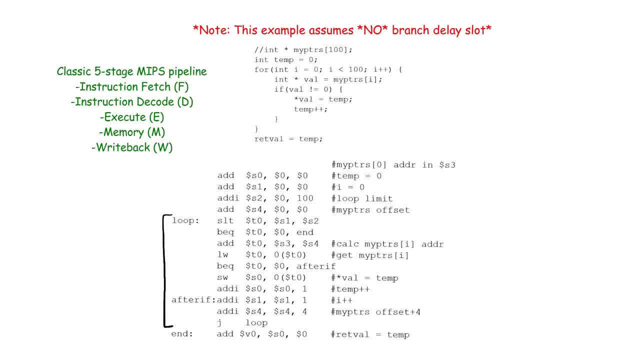 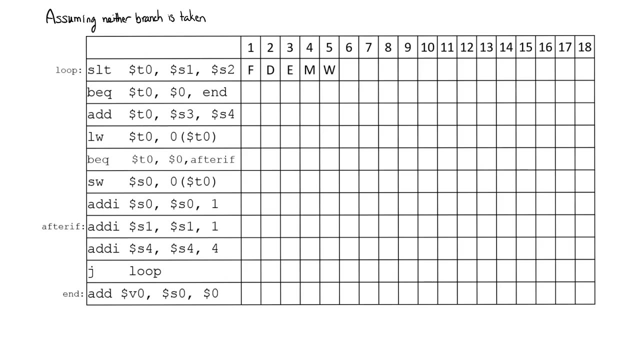 taken exiting the overall loop And we will look at each of these in sequence. This figure is showing each of the 10 instructions in our loop and it's showing cycles horizontally across the top and we're going to look at how each of these instructions proceeds through each of. 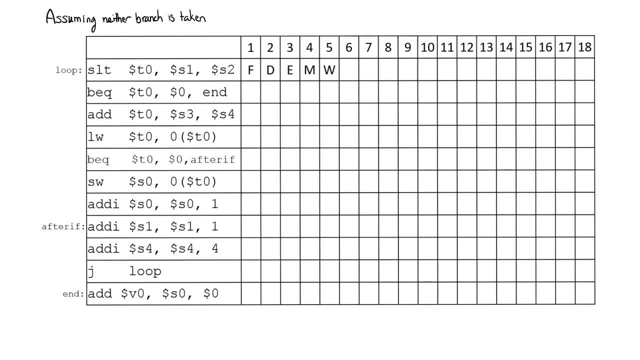 the stages of our pipeline And to start off with- in this case we're going to assume that neither of the branches are taken. We've already shown how the set on less than would basically go through the five stages in sequence. To help with the remainder of the instructions, we want to 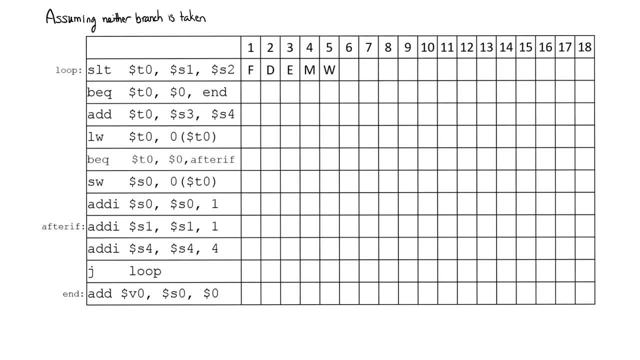 identify any potential dependencies that might force us to stall the pipeline, And so the first thing that we can see is that there is a dependency between the set on less than and the branch on equal. So we're going to use the result for T0 until the end of the execute stage, but the branch on 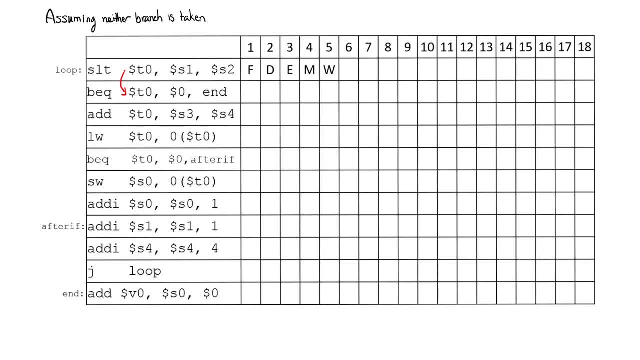 equal needs this result in the decode stage to be able to resolve the branch. There is also a dependency between the add and the load word, but in this case this dependency will be taken care of by forwarding, so we don't explicitly have to stall the pipeline to deal with this. There is also 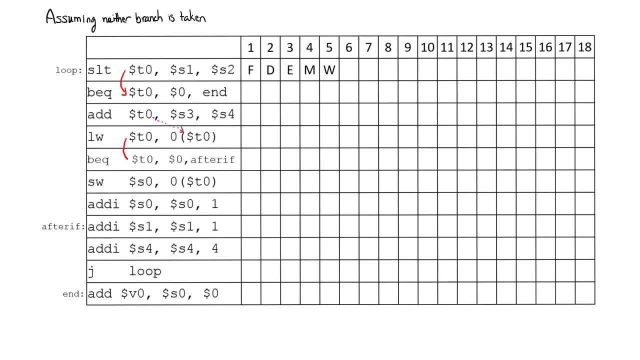 a dependency between the load word for T0 and the branch instruction. The value of T0 is going to be T0 from the load word will not be available until the end of the memory stage, but the branch on equal will need the result or the value for T0 in the decode stage so it can resolve the branch. So 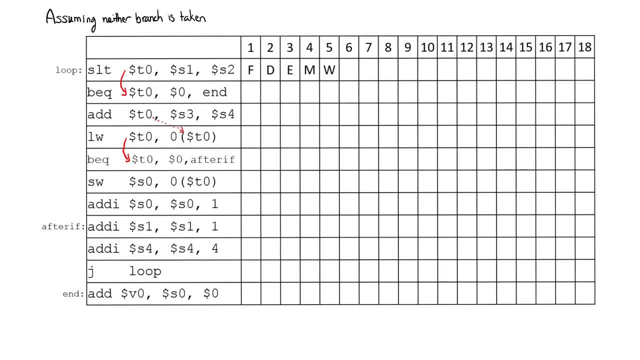 we're again going to need to stall the pipeline And there is also a dependency between T0 of the load word and T0 in the store word. but this is again a case where the implicit forwarding or the natural forwarding we have in the processor will take care of this for us, so we don't have to stall. 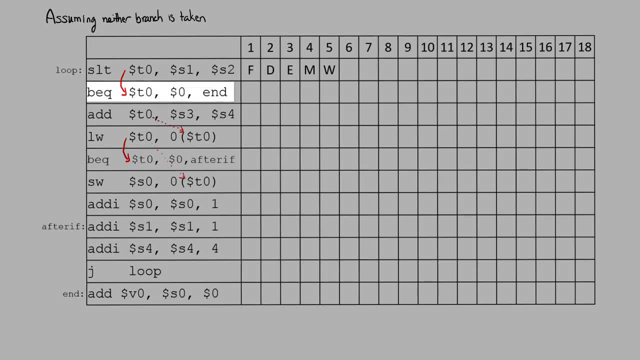 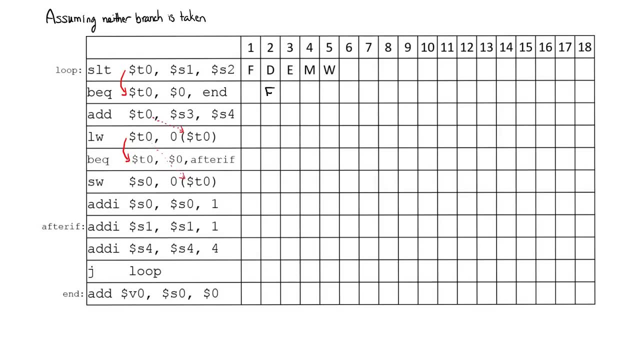 the pipeline. So, going back to our code, we're going to need to install the pipeline. So we're going to need to install our branch on equal instruction at the top. This would start off in cycle 2, in the fetch stage, and then in cycle 3 it would attempt to go on to decode, but it would be. 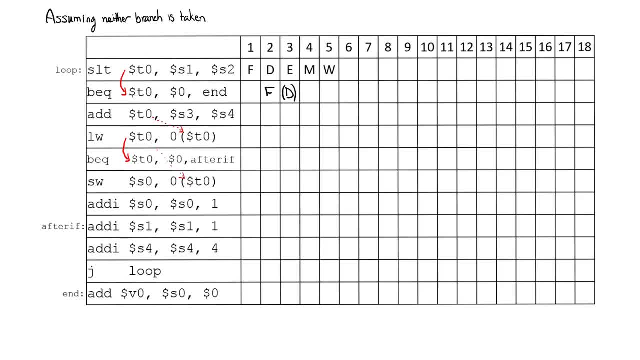 determined that there's a dependency between the set on less than and the branch on equal, since we're looking to be able to forward the value from execute to decode. So we'd have to stall the branch for one cycle and similarly the add would be stalled in fetch and then the branch could go. 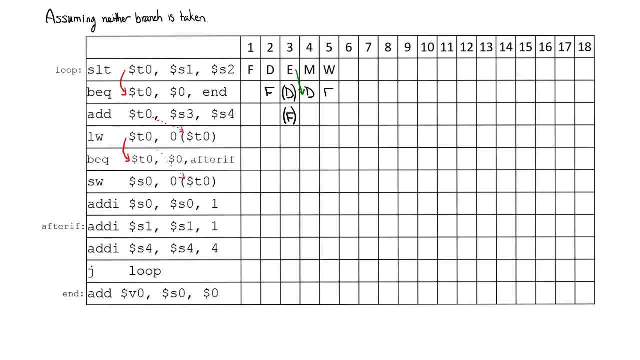 through the remaining cycles. So one cyclone could get its value and similarly the same thing for the add instruction For the load word. there aren't any dependencies that we have to stall for, so we can just proceed through the pipeline like normal. Looking at the branch, it would be first fetched and then the processor. 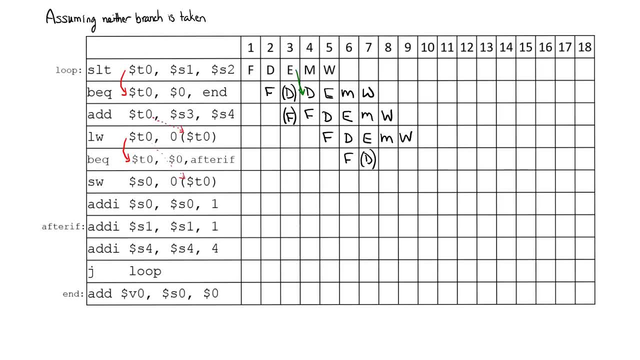 while attempting to decode, would realize that there is a dependency between the load word and t0, and the branch needing t0. And since the load word wouldn't produce the value for t0 until the end of the memory stage, we can't actually perform the decode until cycle 9, so we'd actually 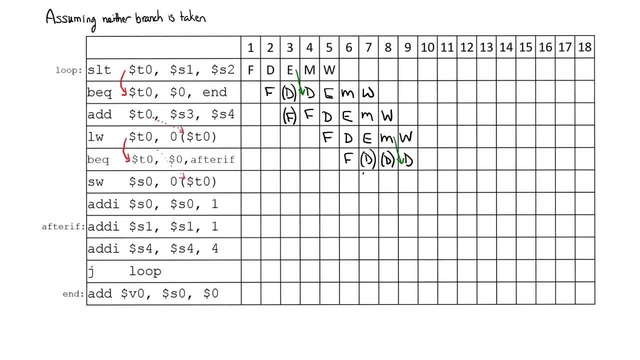 have to stall the branch instruction for two cycles, meaning that the store word would also be stalled in fetch for two cycles, And so then these instructions would complete through the remainder of the stages of the instructions. there aren't any dependencies, so these can proceed through the pipeline. 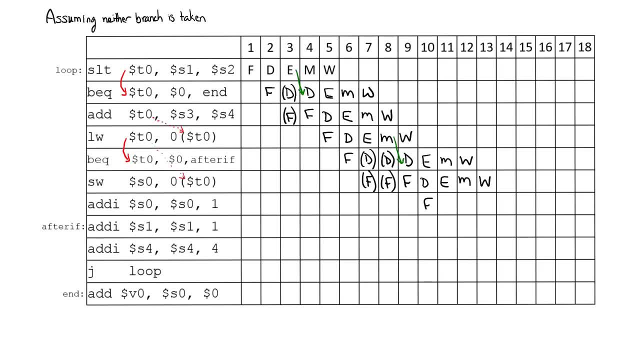 in sequence without any stalls. so they would basically go through the five stages in sequence and then looking at the jump, this is a little bit interesting as well. so the jump would be fetched and then the processor would only realize that it's a jump instruction in the decode stage. but 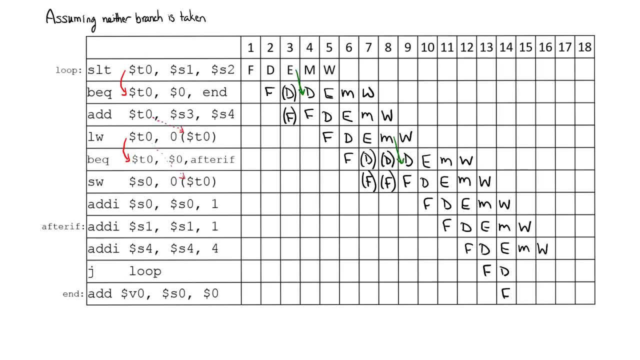 it has already fetched the instruction. after that, and since we're not assuming any branch delay slot, we don't actually want to execute the add instruction, so we want to turn that into a no op while the jump is moving on, and so we've started this instruction unnecessarily and so it's only in. 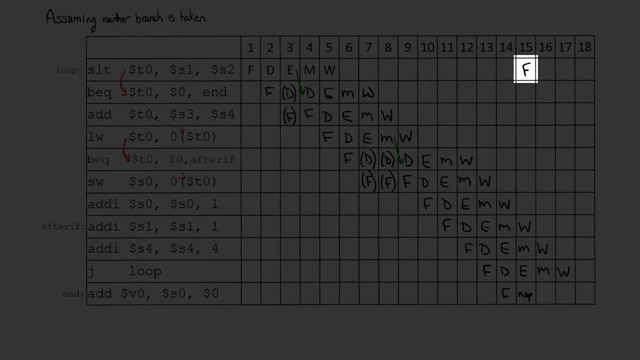 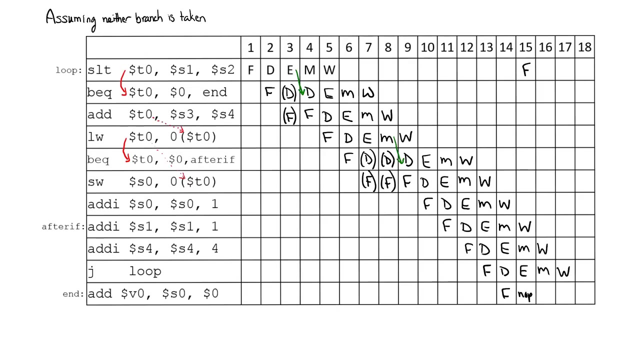 psycho 15 that we'd actually start fetching the set on less than when we start repeating this loop. and then these instructions. one from the repetition of the loop would basically look like this: they did from the start or from the first time, and so this shows how the instructions would execute through the different stages of the 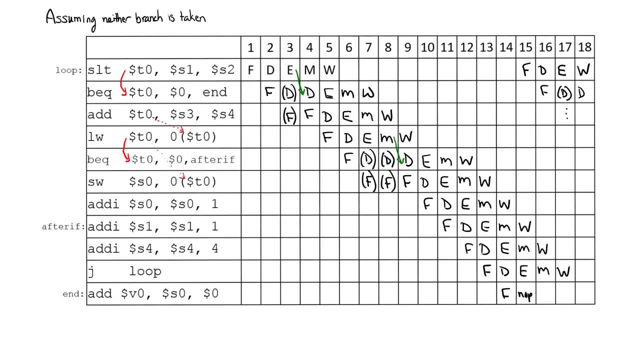 pipeline. often we're also interested in determining how many cycles on average it takes for an instruction to complete in some sequence, and so there's a few ways we could do this. one would be to look at this diagram and try to determine how many cycles it takes between the right back of the first instruction. 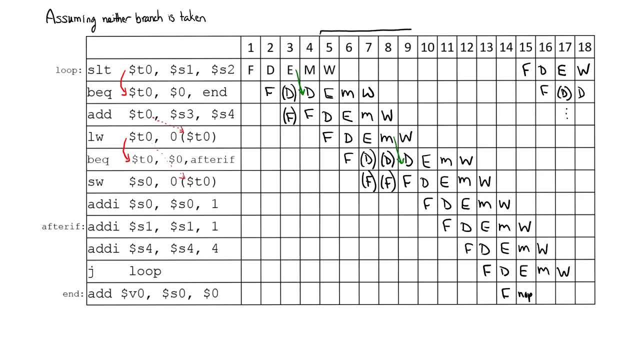 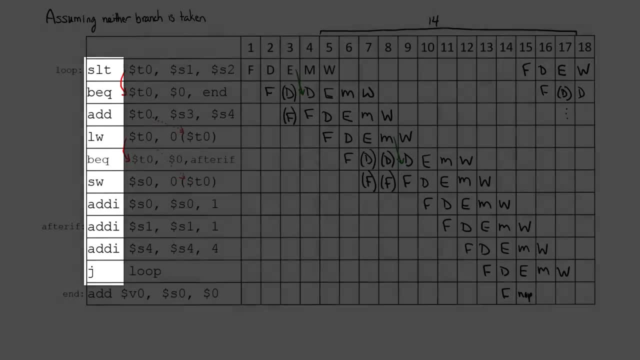 and the left back of the second instruction, so we could see in this case that one iteration spans this many cycles, which ends up being 14 cycles, and if we counted it out, we could see that there are also 10 instructions in this loop that we're executing that we actually want. 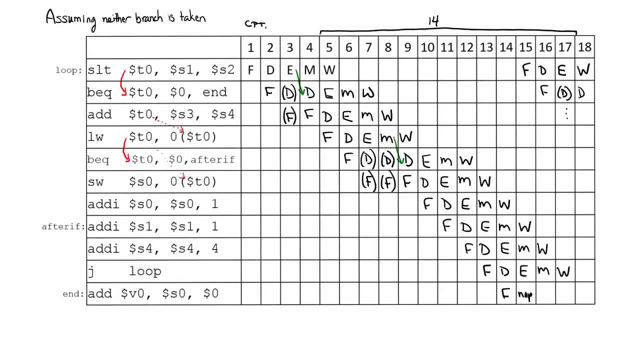 to happen, and so one way we could calculate the cpi would be to say that we've got 14 cycles that we're spanning over, and we said there were 10 instructions, and so this would give us a cpi of 1.4. an alternative approach would be to look at the individual instructions and 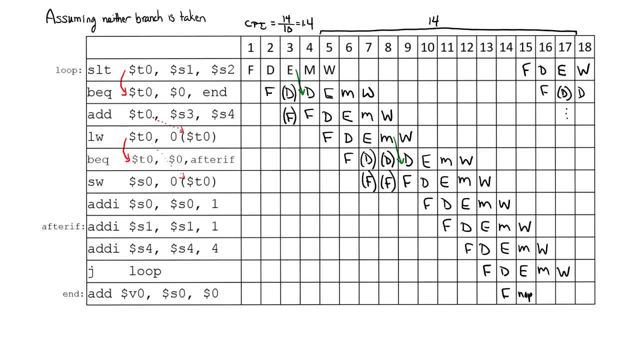 see how many cycles they consume on average. for example, the set on less than doesn't have any stall, so in the steady state case this basically just takes the equivalent of one cycle, because there are other things happening in parallel and so we're only interested in the one cycle it takes. 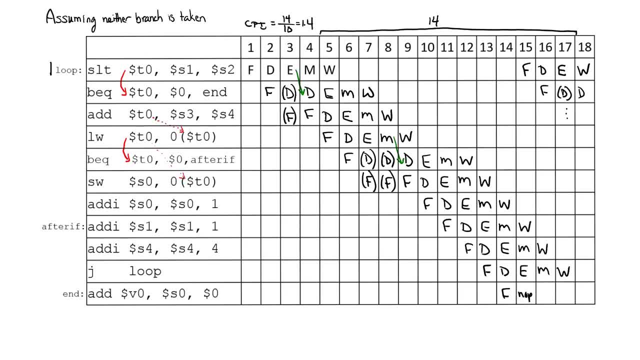 for the right back for the branch instruction, since it had to stall, this takes the equivalent of two cycles to complete. the add doesn't have any explicit stalls for itself, so it's only one cycle and the same for the load word. the second branch instruction actually actually has to stall for two cycles. 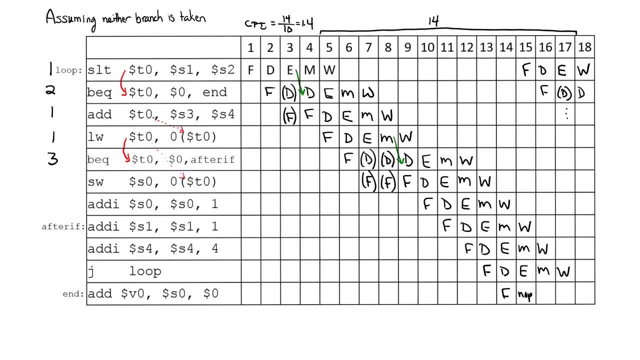 so it consumes the equivalence of three cycles per iteration. the store doesn't stall, and neither do any of the add immediate instructions and then the jump. while it doesn't stall, it appears to take the equivalent of two cycles because the instruction after it starts to be executed and then has to be squashed, and so we can kind of consider this as taking two. 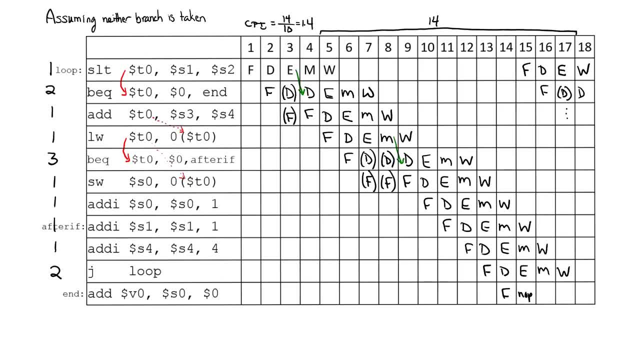 cycles, and so if you add all of these up, you'll also come to the fact that we've got 14 cycles going on here, and so we could also calculate the cpi the same as we did before. if we added up all these numbers and divided by our 10 instructions, we'd also get 14 over 10 or the 1.4- another case. 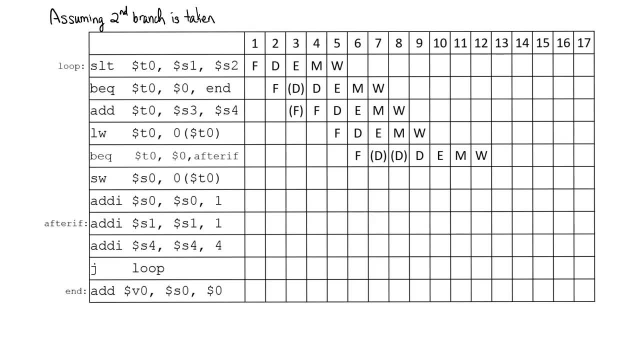 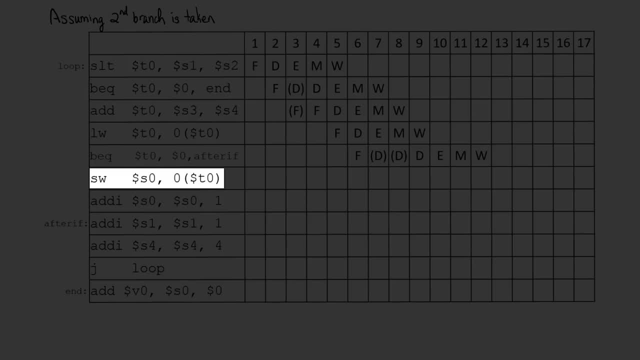 of interest when the second branch is taken, and so that means the first five instructions would execute just like they did the first time through, and it's only when considering the instructions after the branch that things would change. and so, looking at the store word after the branch, if the branch is going to be taken, this 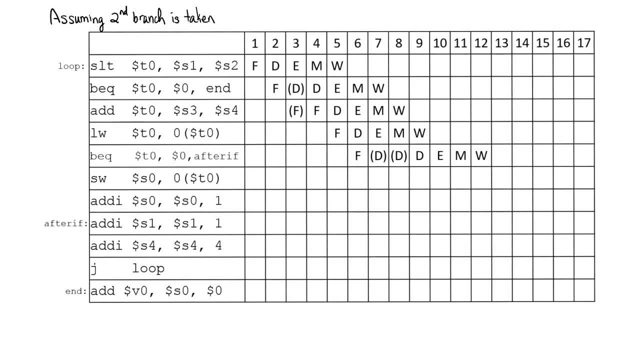 means that the store word is not really going to be executed. but we don't find this out until the end of the decode stage. so the store word would start to be executed, so it would be fetched, and it would be only at the end of the decode stage for the branch or going into the decode stage for the store word. 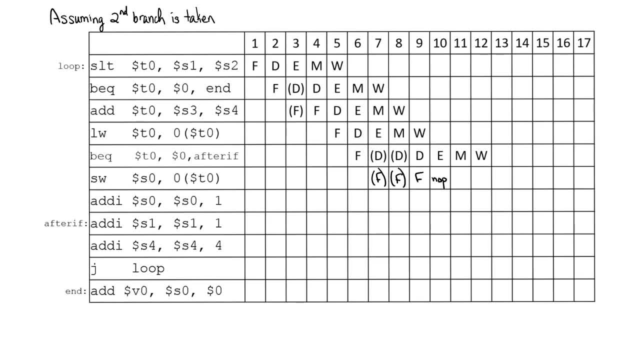 that it would be realized that this instruction actually shouldn't be executed and would be turned into a no op, and so it would be in that same cycle, cycle 10, that we'd actually jump to the after if place. so we'd start fetching the add immediate, and since there's no dependencies here, this would: 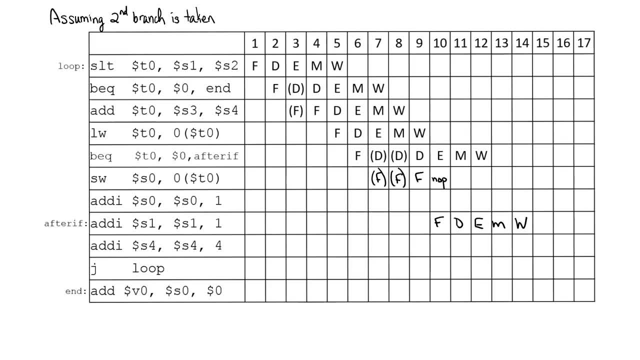 continue through all its typical cycles, and then we would continue through the remaining instructions. we did in the case where we had none of the branches taken, and so this would mean that the issue or the execution of the jump where the second instruction or the instruction after it starts to execute, would still happen. 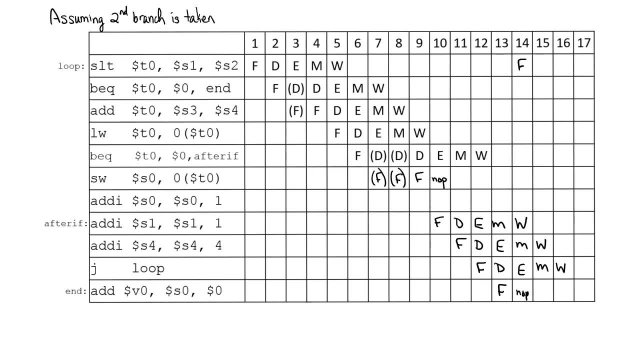 and so in this case the set on less than instruction would start in cycle 14 as opposed to cycle 15 and would continue through just like it did the first iteration, and so when evaluating the cycles per instruction in this case, we could again take either of the. 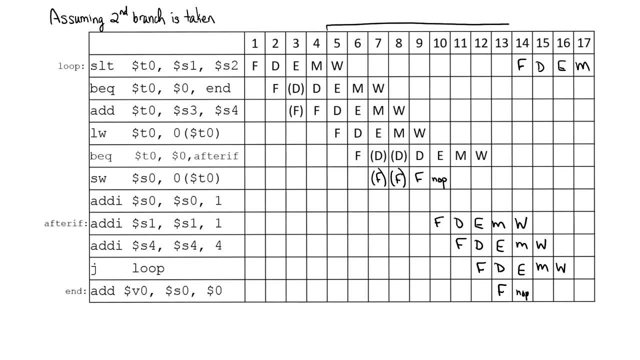 two approaches. we could look at counting from 5 to 17 here, where we find there are 13 cycles, or we could also look at the individual instructions and determine how many cycles they take on average or they appear to take. so the set on less than would still be one. 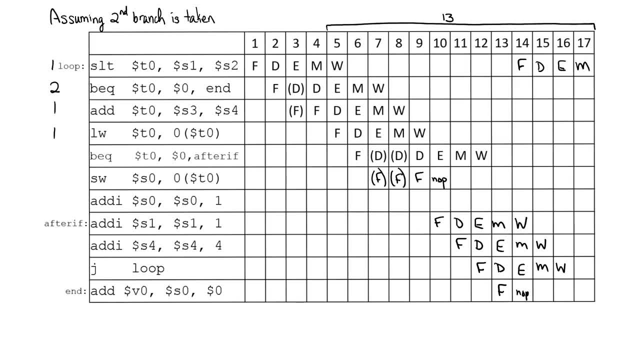 the branch from before would be two, one one, and then for this second branch, not only is it going to take two additional cycles for the two stall cycles, it's also going to have to account for the fact that it had to squash the store- word instruction- and so it would have the equivalent of taking four cycles, and then the two add. 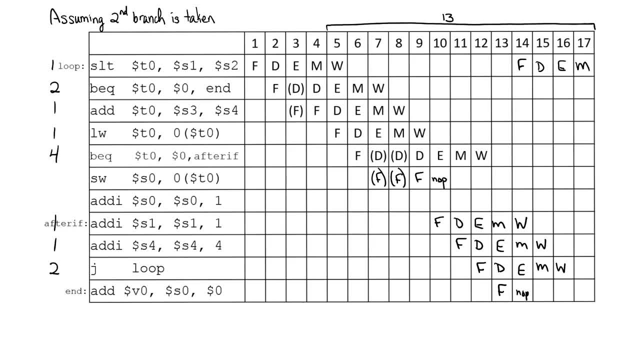 immediates would take one and the jump would take two, as before, and so, adding these up, we would again find that we had 13 cycles, and so the cpi in either case would have 13 cycles, and in this case, since we're not executing two of the instructions, we're 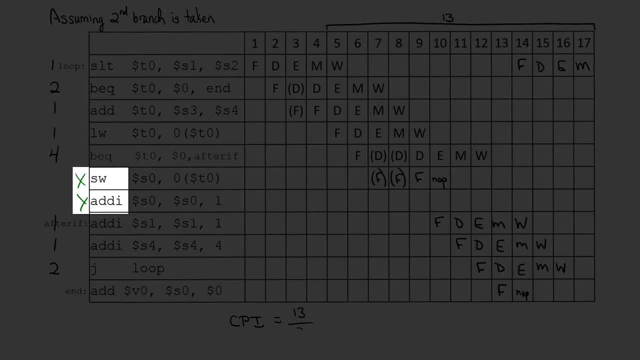 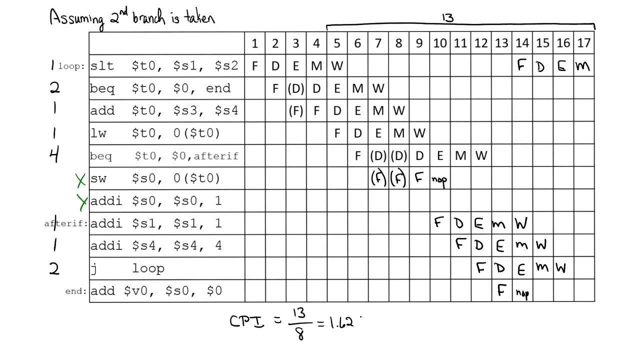 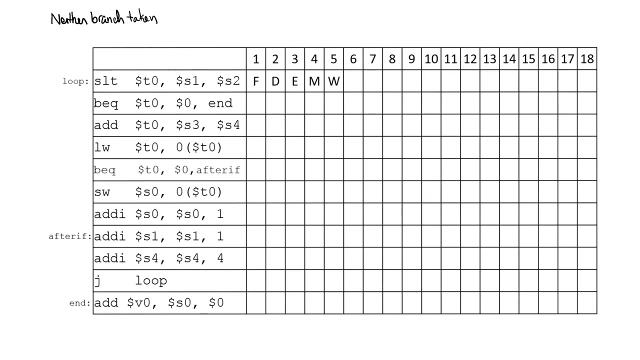 not executing either of these two instructions. we really only have eight instructions that are being executed, and so this gives us a CPI of 1.625.. The final case to consider is when neither of the branches are taken, and so basically, that means that it would be this top branch that is the one that 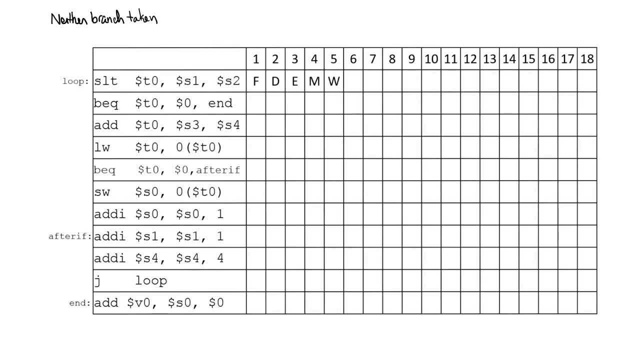 would exit the loop, and so this would only happen on the very last time, and so in this case we fetch the branch, we'd have to again install the decode while we wait for the value of t0, and then, in cycle 4, we'd be able to decode the. 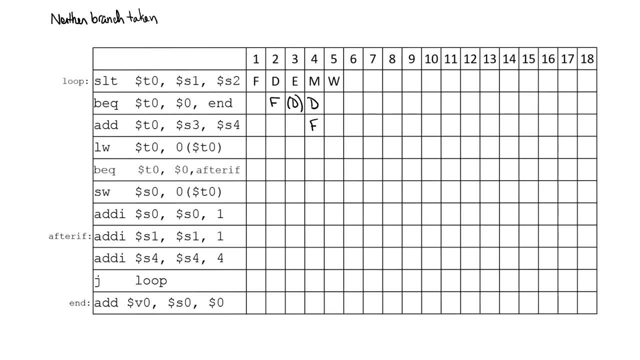 branch, but at the same time we'd start to fetch the add instruction, and it would only be at the end of cycle 4, as we're going into 5, that we'd realize that the branch is being taken and we're leaving this loop. and so it's only at 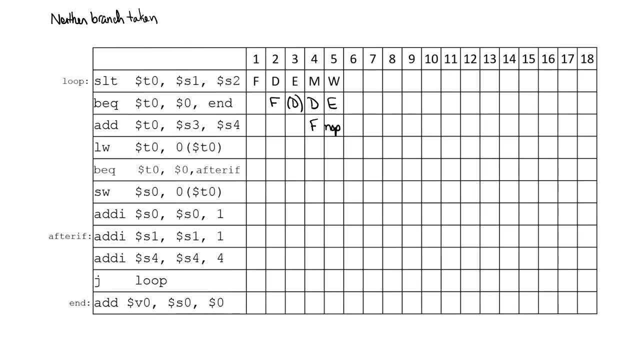 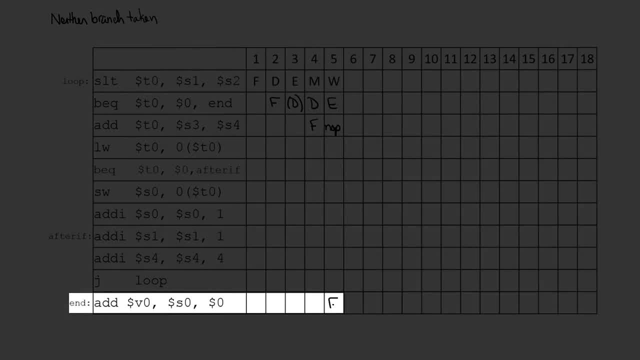 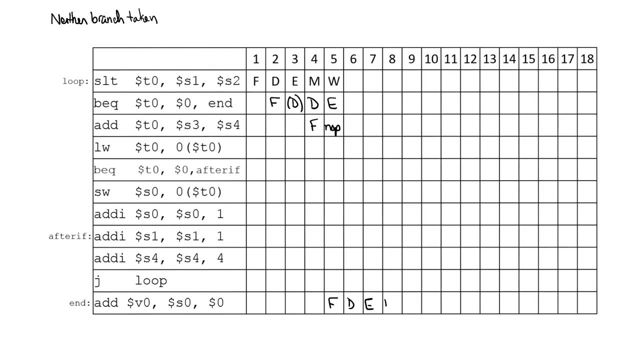 this point that we branch out, and we would turn this fetched add instruction into an OOP and then basically, we would come down to the end and we would start fetching down here at the end, and so these would go through typical stages and the same thing for the branch instruction, and so that's all that would happen. when neither 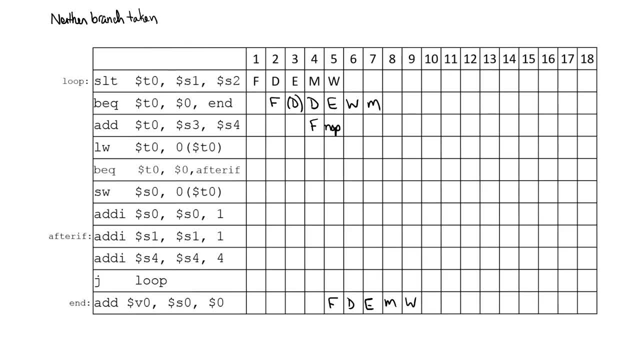 branch is taken. Looking at the number of cycles per instruction on average when we're exiting, focusing just on the two instructions within the loop and not on the instruction that happens outside of the loop, we can see that the set on less than is still taking one cycle and in 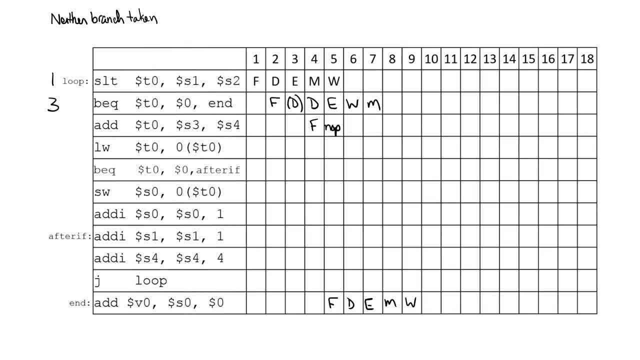 this case we would consider the branch to be taking the equivalent of three instructions, because it has the one cycle due to the stall from the decode and then an additional cycle due to the squash of the add instruction and turning that into an OOP, and so the overall CPI in this case would be the 1. 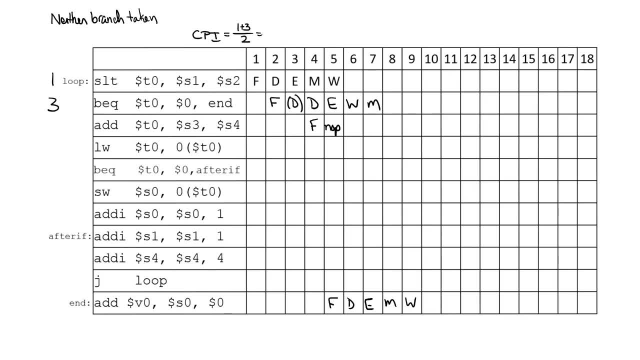 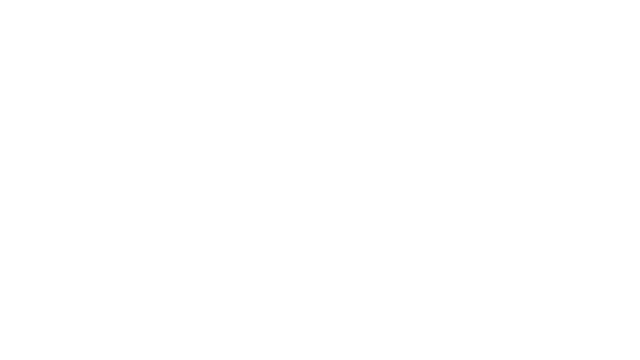 plus 3 and then divided by two instructions, or 4 over 2 or 2.. With these three pieces in place, we're interested in looking at the CPI of an entire execution of this loop. So we're interested in the overall CPI for some execution. 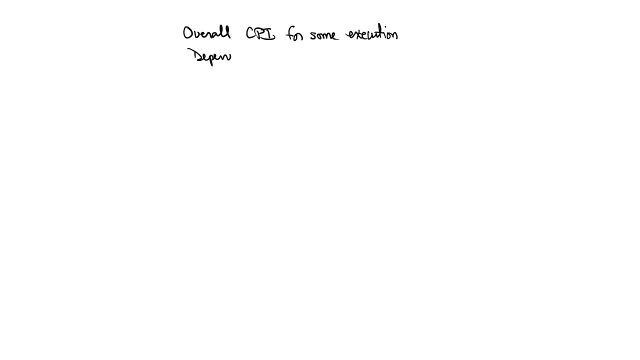 and what the CPI actually depends on the actual behavior of that branch to time that the нас point table targets. we're interested in pouching overall STO of the an t into all those CDT and, madame this, hundred iterations of the loop plus the exit. and so we is one way to 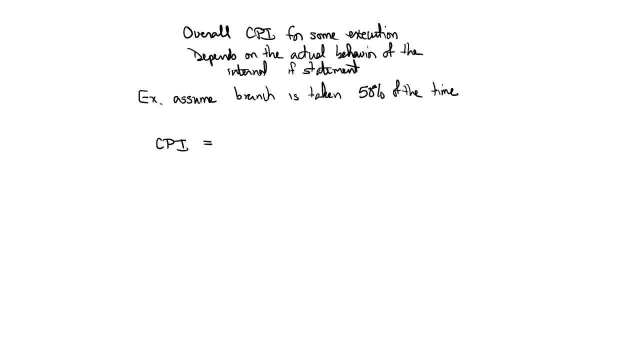 consider this, or to look at this, would be to consider the 50 cases when the branch is not taken, the 50 cases when it is taken, and then the final exit. and so, looking at the case, the 50 cases when it is not taken, in this case, all 10. 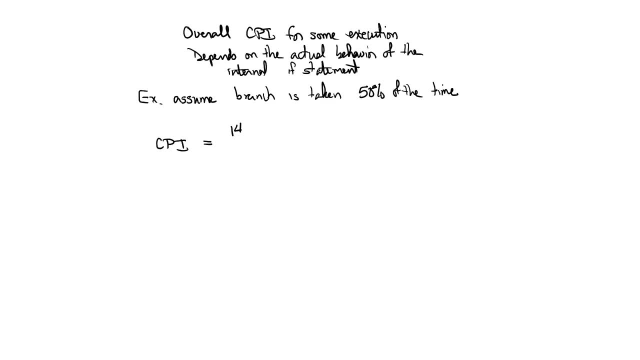 instructions are executed and we previously found that it took 14 cycles and there were 10 instructions, and we're assuming this happens in 50 of the 100 cases. so that's one portion for the 50% of the time or the 50 iterations. 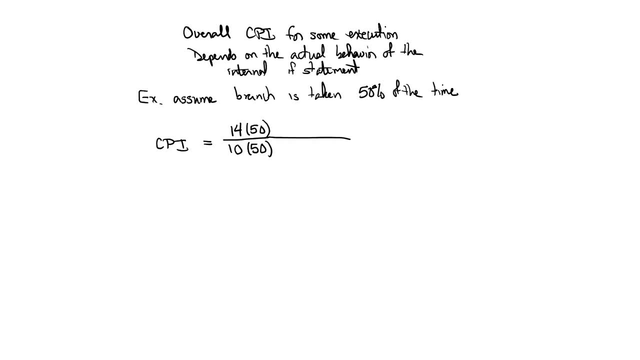 where the branch is taken, meaning that the if isn't executed. we found that there were 13 cycles for this and that there were eight instructions executed. and then, finally, to exit the loop, we found that it took four additional cycles and two additional instructions to do the last set on less than and the 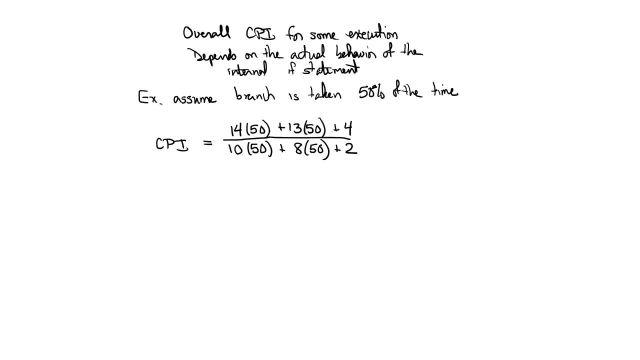 last branch, and so if you calculate this all out, you find that this is approximately equal to 1.5. so this loop, executed a hundred times, had an average CPI of 1.5.